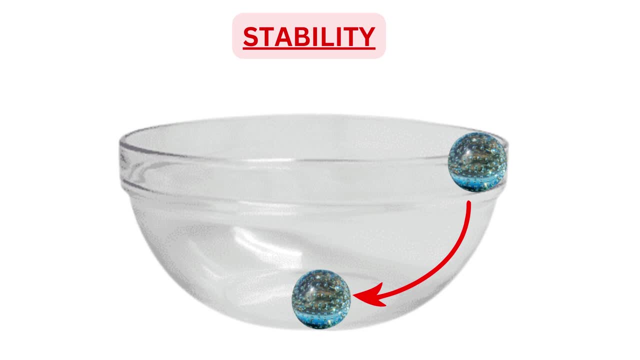 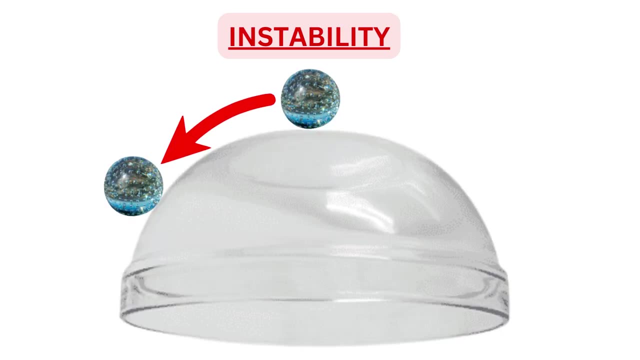 property is called stability, The property of an object to return back to its original position. Now take another example. Keep the bowl inverted and once again keep the glass ball on top of it. Apply a sideways force on the glass ball and leave it, This time instead of returning to original position. 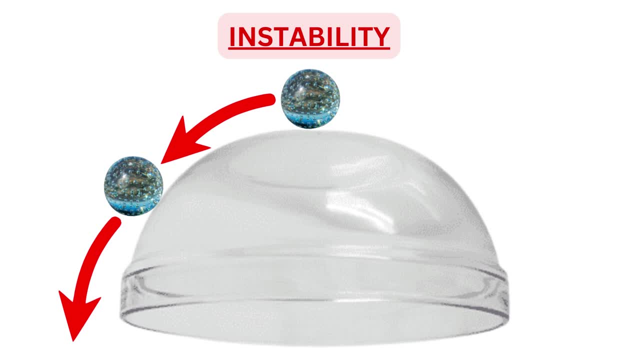 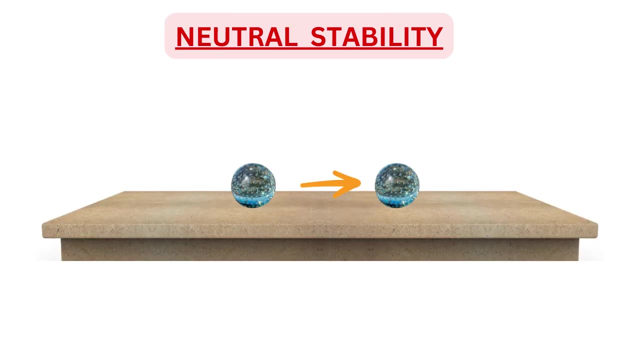 the glass ball will continue to move away and finally fall down on the ground. This is called instability- Property of an object to continue moving away once displaced from original position. And the last is neutral stability. To understand this, just keep the glass ball on the horizontal table. Slide the glass ball. 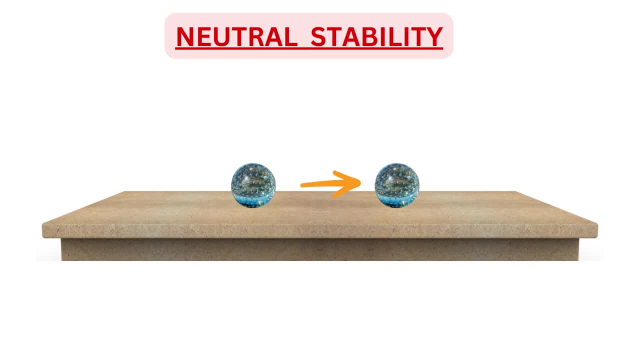 to any side and leave it. In this case, the glass ball will neither move back to original position nor will it move away, but it will remain at the last position where it was left. This is what is called neutral stability. So, having understood the stability now, we are ready to understand the atmospheric stability. 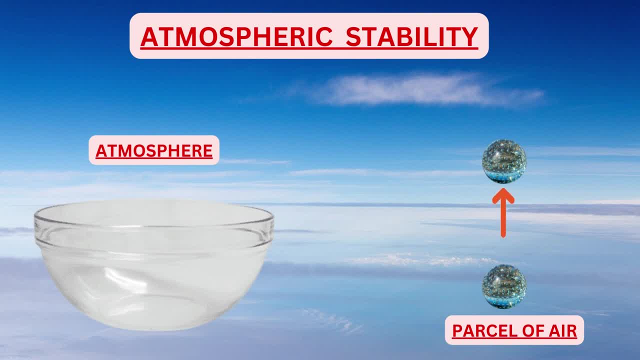 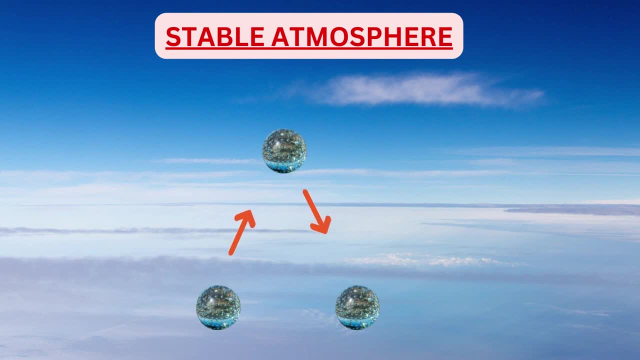 Here the bowl is the atmosphere and the glass ball is a parcel of air which has been forced to move vertically upwards. If this parcel of air comes down when the force is removed, then it is a stable atmosphere. If it continues to move further upwards, then it is unstable. 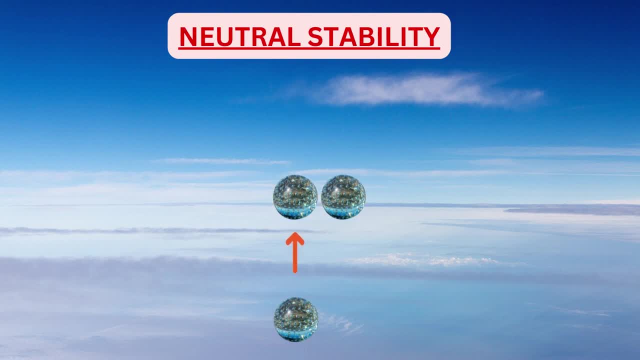 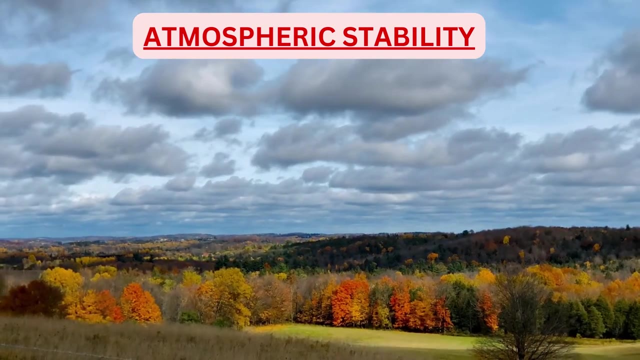 atmosphere and if it remains at the same location where it was last left, then it is neutral stability in the atmosphere. So in this chapter we will discuss the weather conditions which govern whether the atmosphere at a given place and height is stable, unstable or neutral. 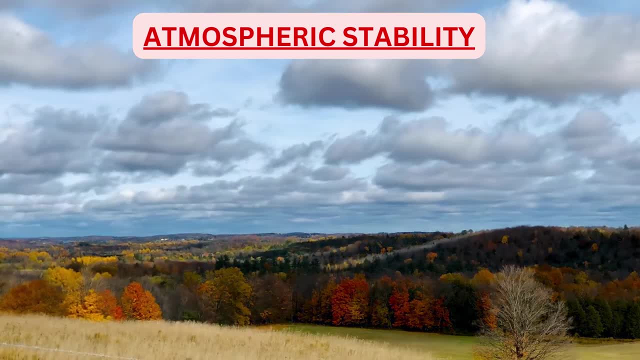 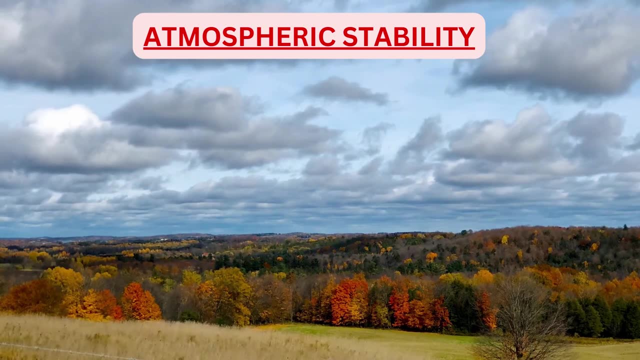 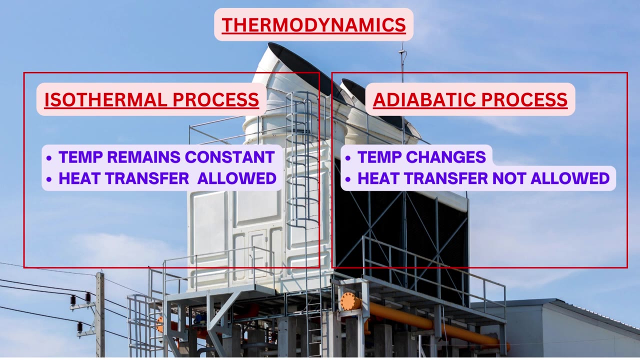 Atmospheric stability governs the weather conditions in that geographical area. To understand this subject with clarity, we need to understand one more term of physics, which is called adiabatic process. In thermodynamics, there is isothermal process and adiabatic process- Iso thermal process. 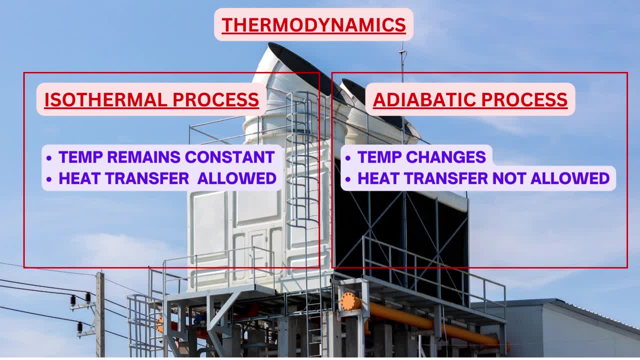 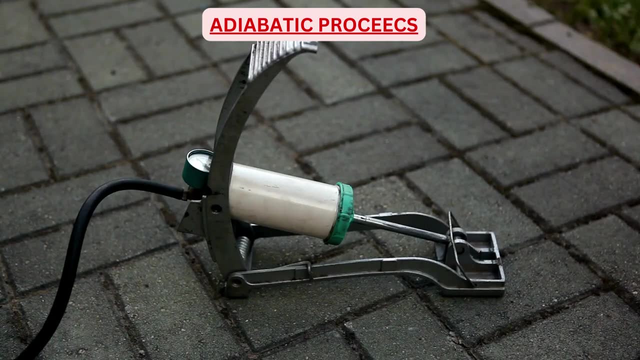 is one where the temperature of the system remains constant, since heat is allowed to be transferred out of or into the system. In the adiabatic process, temperature changes since the heat is not allowed to enter or leave the system. Example of adiabatic process is filling of air in bicycle. 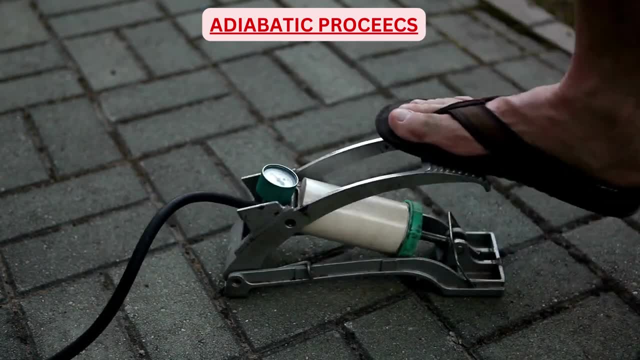 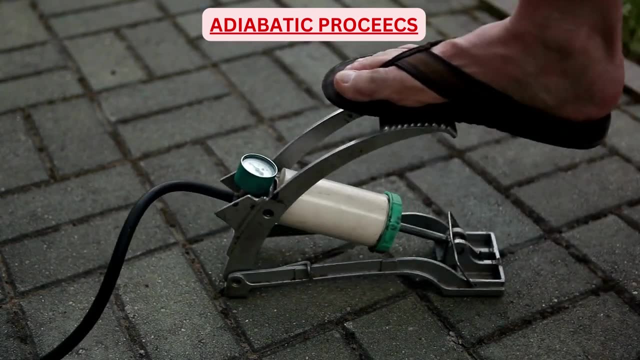 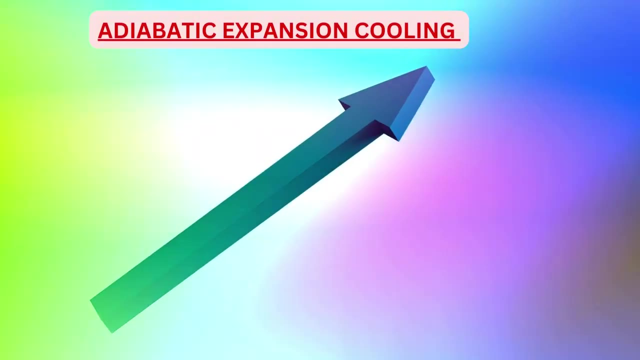 with a manual pump. The pump gets heated up due to the compression of air. So in adiabatic process the compression results in heating and expansion results in cooling. Now in atmosphere, when a partial of air is forced to move upwards atmospheric pressure, 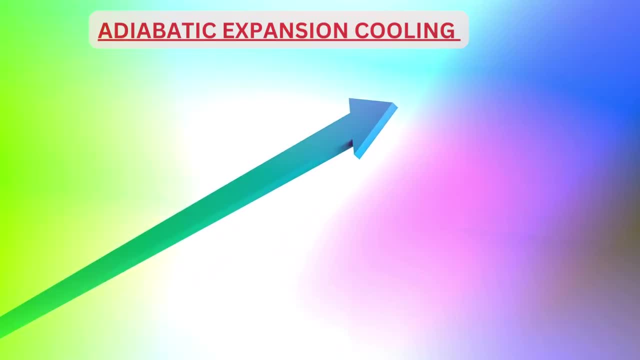 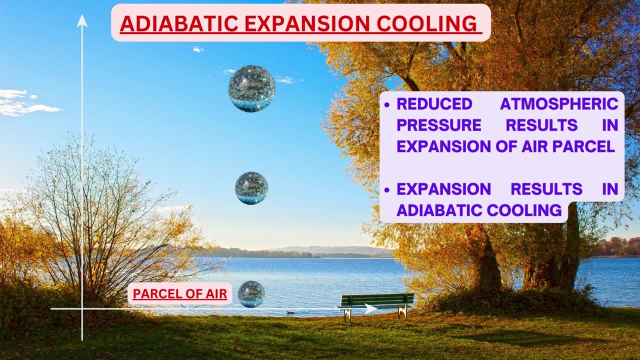 exerted on this partial of air keeps reducing, Since you know that the pressure or atmospheric pressure reduces with increase in height. So there is expansion of this partial of air as it moves upwards and this expansion will result in adiabatic cooling. Thus, a partial of air which 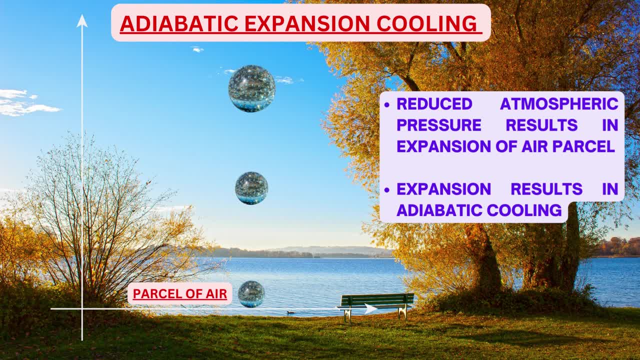 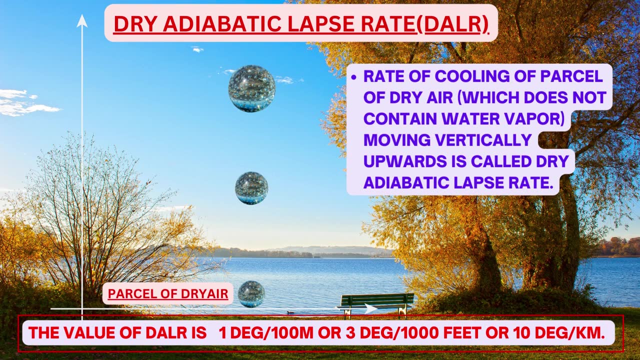 is forced to move upwards will always cool down due to adiabatic expansion cooling. And remember this cooling effect is purely due to adiabatic expansion and not because of the environmental lapse rate. Dry adiabatic lapse rate- DALR- The rate of cooling of a partial of dry air which does not contain 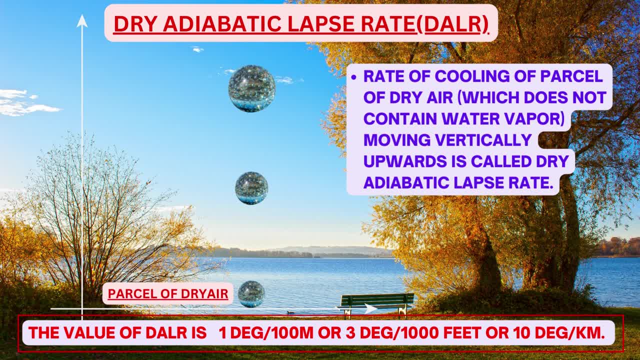 water vapor moving vertically upwards is called dry adiabatic lapse rate And the value of dry adiabatic lapse rate is 1 degree per 100 meter or 3 degree per 1000 feet or 10 degree per kilometer. 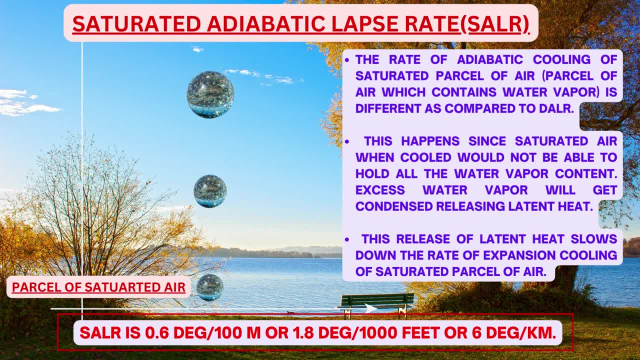 DALR- saturated adiabatic lapse rate. The rate of adiabatic cooling of saturated partial of air, a partial of air which contains water vapor, is different as compared to DALR. This happens since the saturated air, when cooled, will not be able to hold all the water vapor content. 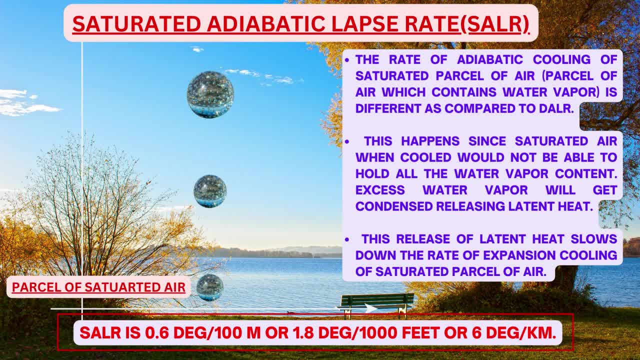 Excess water vapor will get condensed, releasing latent heat, And this release of latent heat slows down the rate of expansion. cooling of saturated partial of air. Of course, SALR will be lesser than DALR and the value of SALR is 0.6 degree per 100 meter. 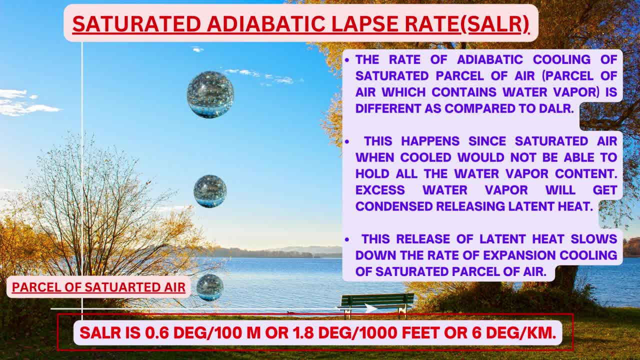 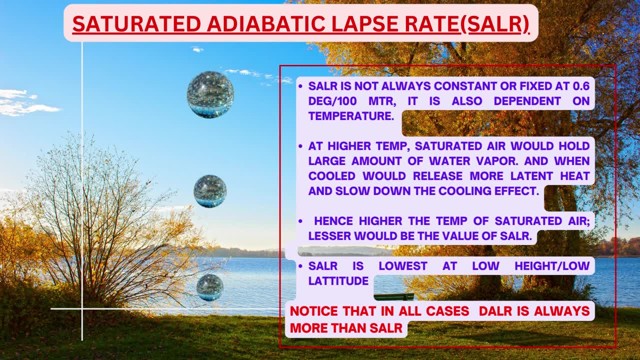 or 1.8 degree per 1000 feet or 6 degree per kilometer. Salr is not always constant or fixed. at 0.6 degree per 100 meter It is girls plus 6 degrees et permit鈨. 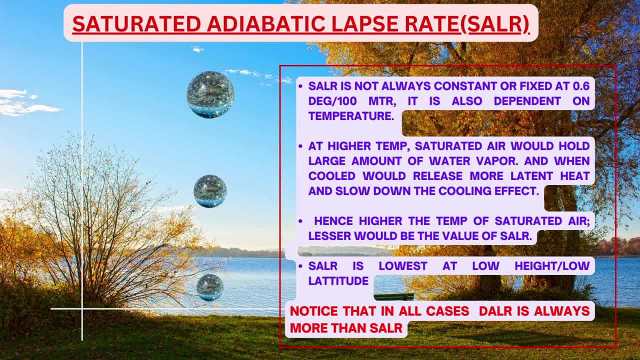 manuel Culture, NYC��Turk tropicclr websiteуєxpresscom foranyam subscribers crossing theDIR. dependent on the temperature. at higher temperature, the saturated air would hold large amount of water vapor and when cooled will release more latent heat. and 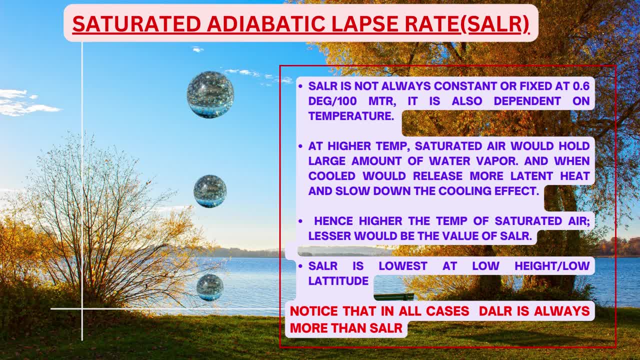 slow down the cooling effect, hence higher the temperature of the saturated air, the lesser will be the value of salr, and salr is lowest at low height, since the temperature is higher at low height, and slr is lowest at low latitudes, since at lower latitudes the temperature is higher. and notice that in all cases the 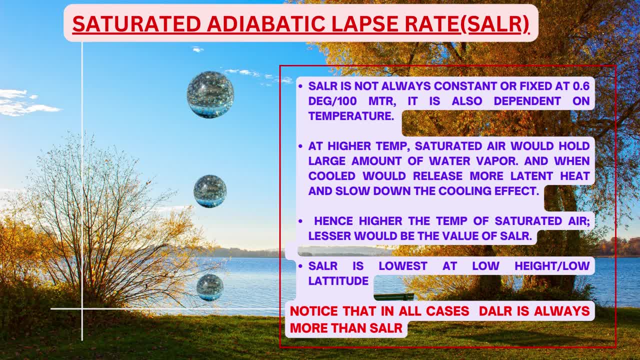 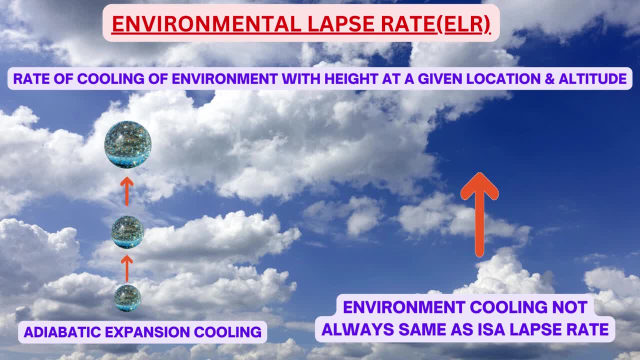 dalr is always more than salr. elr. environmental lapse rate. we have studied in lesson 1 of metrology that as per international standard atmosphere the sea level temperature is plus or minus 1 degree Celsius and the temperature is plus 15 degree and the temperature reduces with height at a rate of 6.5. 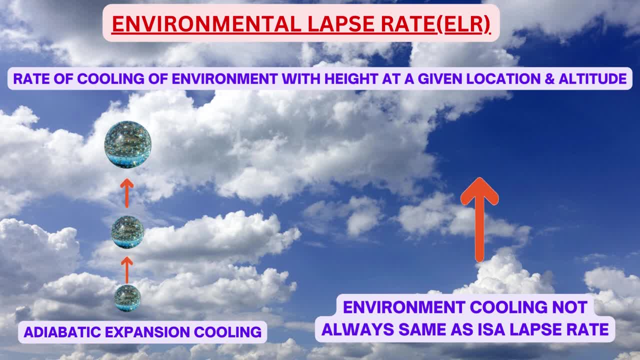 degree per kilometer till tropopause. this is called temperature lapse rate in atmosphere. but this ideal condition may not and will not exist everywhere and every time. in real world, at different geographical location on earth, at different altitudes, the temperature lapse rate will not be same as ideal. 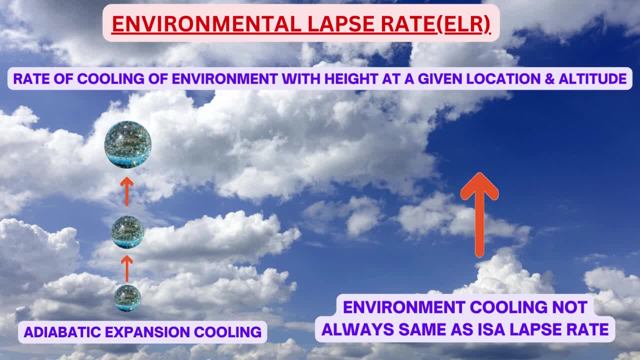 conditions. so this real-world lapse rate is what is called environmental lapse rate or ELR. ELR will govern that when a partial of air is moved to, forced to move upwards, the environment around this partial of air is cooler, hotter or at the same temperature, which will further decide the future path of this partial. 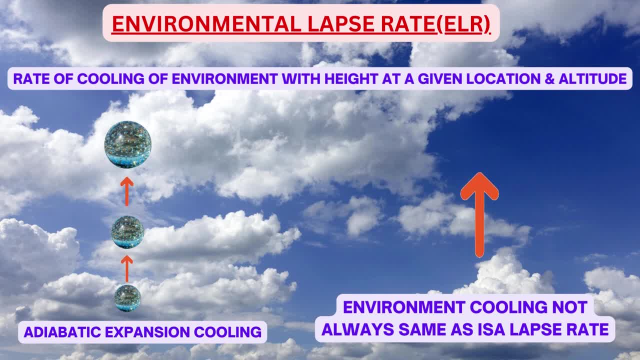 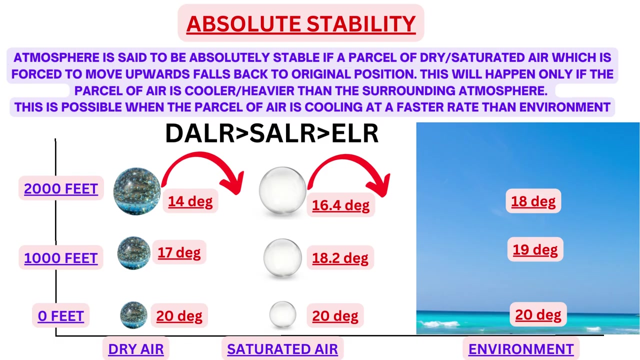 affair and Finally it will decide the atmospheric stability or instability. More or less DALR and SLR values are fixed. It is the ELR which varies with place, time, altitude and latitude. Now let's discuss one by one the conditions for atmospheric stability. 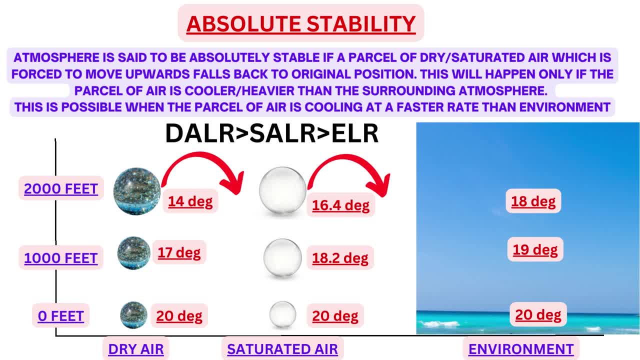 First is absolute stability. Air is said to be absolutely stable if a parcel of dry or saturated air which is forced to move upwards falls back to its original position. This will happen only if the parcel of air is cooler or heavier than the surrounding atmosphere. 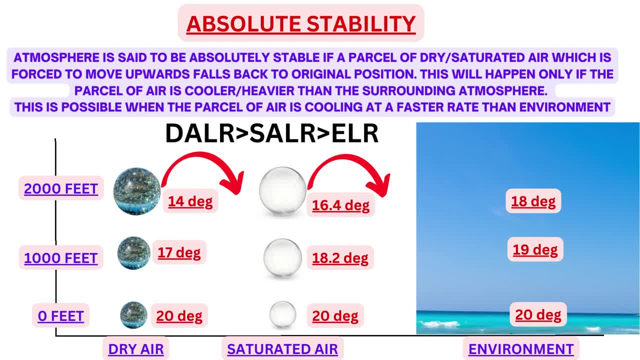 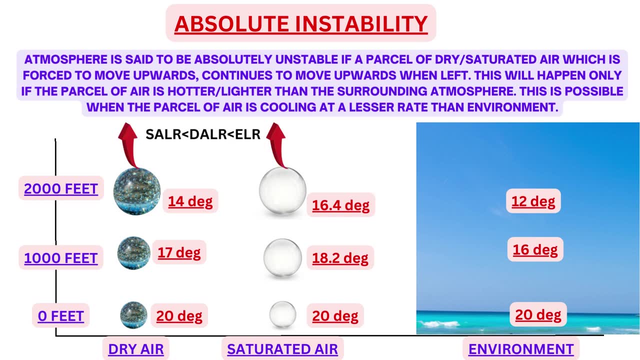 And this is possible when the parcel of air is cooling at a faster rate than environment. or you can say the condition will be DALR more than SLR and SLR more than ELR. Next is absolute instability. Atmosphere is said to be absolutely unstable if a parcel of dry or saturated air, which 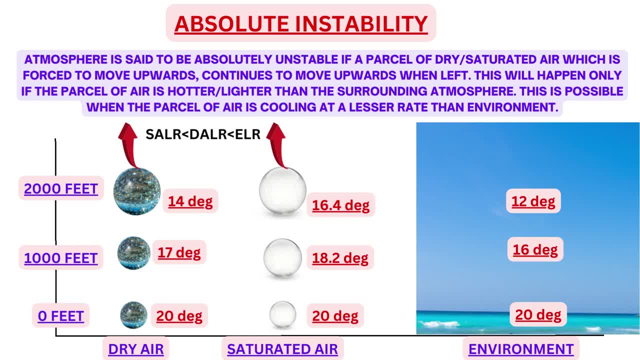 is forced to move upwards, continues to move upwards when it is left. This will happen only if the parcel of air is hotter or lighter than the surrounding atmosphere, And this is possible when the parcel of air is cooling at a lesser rate than the environment. or you can say: 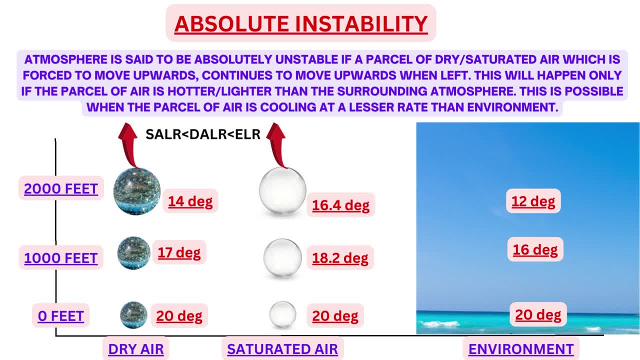 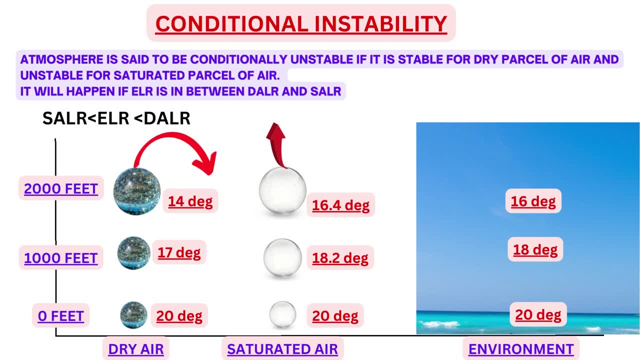 SLR is lesser than DALR and DALR lesser than ELR. Conditional instability: Atmosphere is said to be conditionally unstable if it is stable for dry parcel of air and unstable for saturated parcel of air. and by now you can understand that it will happen. 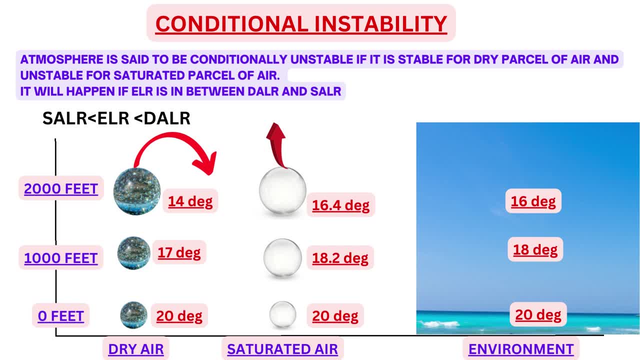 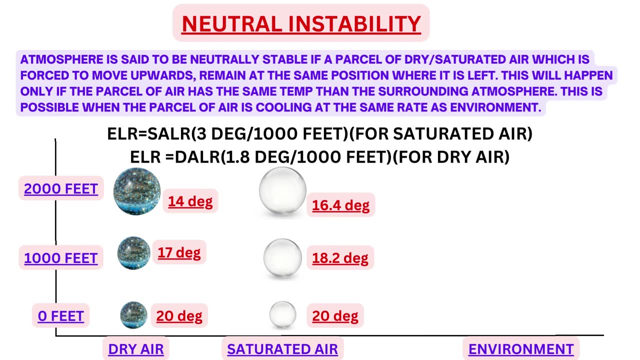 if ELR is in between DALR and SLR, So the conditional instability will prevail. when DALR is more than ELR, more than ELR and ELR is more than SLR, Neutral stability Atmosphere is said to be neutrally. 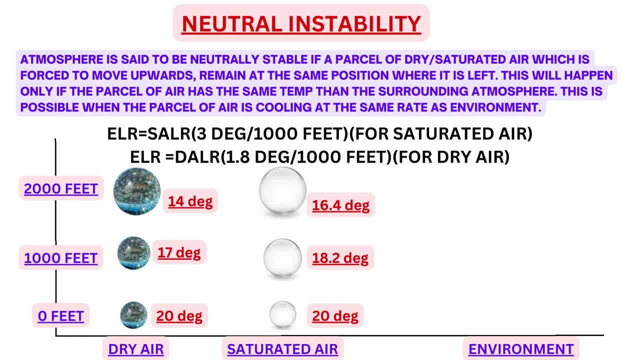 stable if a parcel of dry or saturated air which is forced to move upwards, remain at the same position where it is left. This will happen only if a parcel of air has the same temperature than the surrounding atmosphere, and this is possible when the parcel of air is cooling at the same.